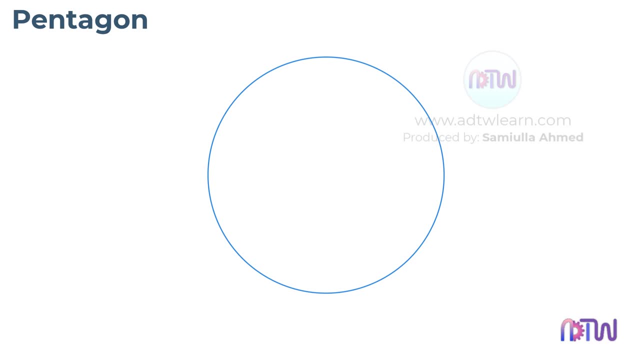 After this, we need to draw a horizontal line passing through the center of this circle. Label these points as A and B and this center point as O. Since we want to draw a pentagon, we need to divide this horizontal line AB into 5 equal parts. 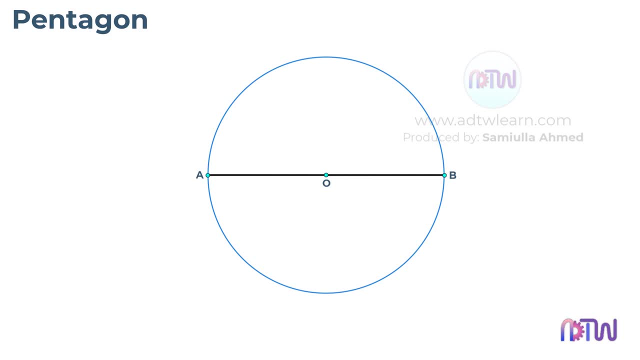 To divide this line into 5 parts. we will draw an inclined line from this point. Take a compass and adjust it to some length and cut 5 arcs on this inclined line. Create a circle. With this shape, we can draw a circle and a vertical line. 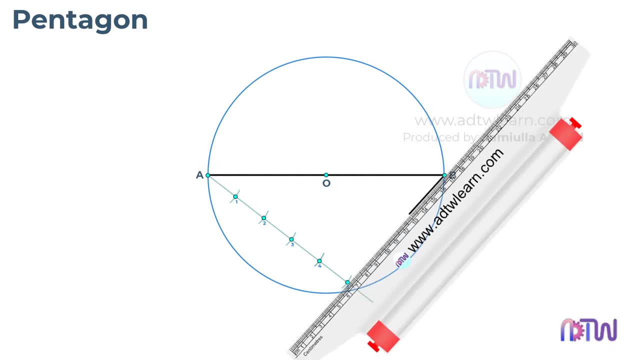 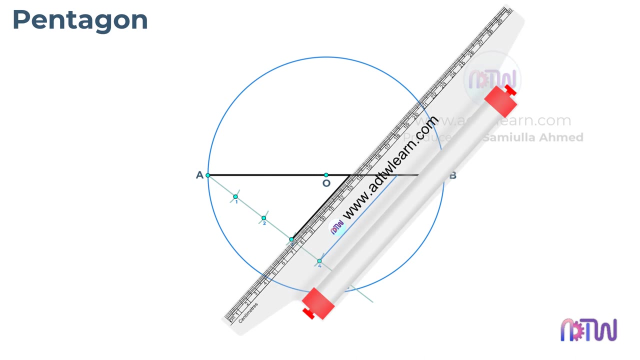 After this, use a drafter or a roller scale to join these endpoints together. Similarly, draw parallel lines to this initial line at each of these points on the inclined line. Draw a parallel line to these points on the inclined line. Do the naming for these points. 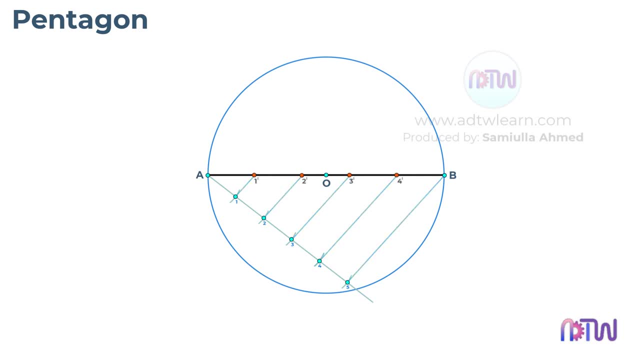 points one dash, two dash, three dash and four dash, Since we divided the line into five equal parts. after this, take a compass and adjust its length to line AB. With this length on the compass, draw arcs above this line AB using points A and B as centers. 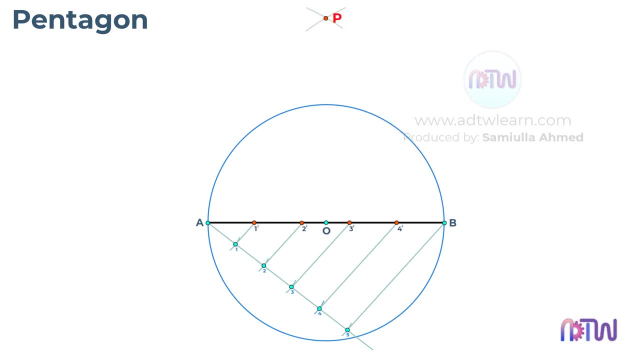 Label this point as P. Next, draw a line passing through this point P and point 2 dash such that it touches the circumference of the circle. This point will be our point C. The distance between point A and point C is the side length of a pentagon, which will 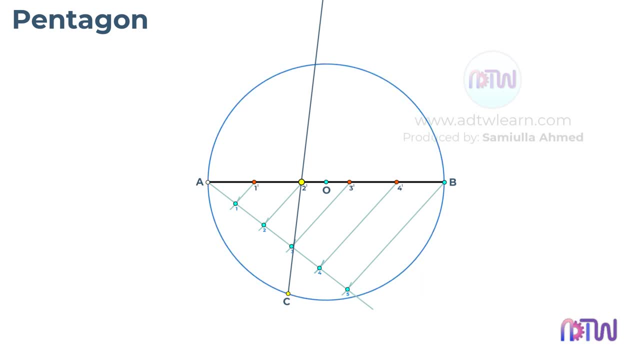 exactly fit into this circle. Using this length, cut an arc on the circumference of the circle. Take a compass and adjust it to this length. AC: Cut arcs on the circumference of the circle. These are the five required points. Subtitles by the Amaraorg community. 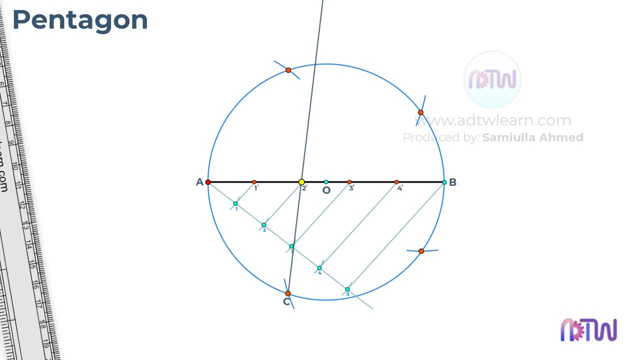 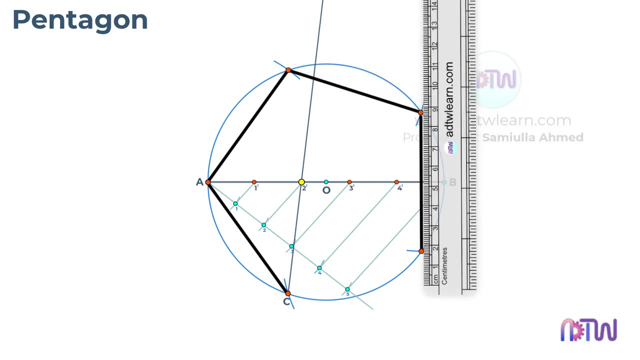 This is our final pentagon. I hope this video helped you in learning something new. If so, click on the like button and if you are new to ADTW, Learn, click on the subscribe button and turn on all the notifications so that you get all my latest videos.